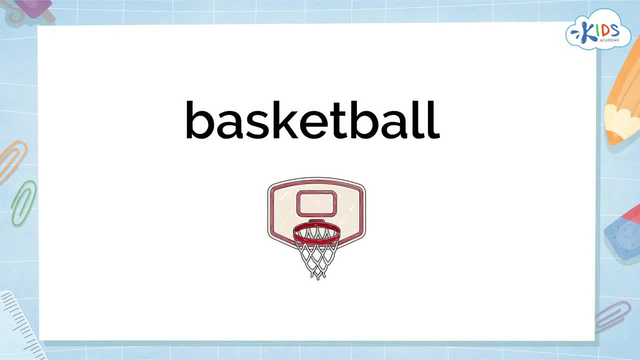 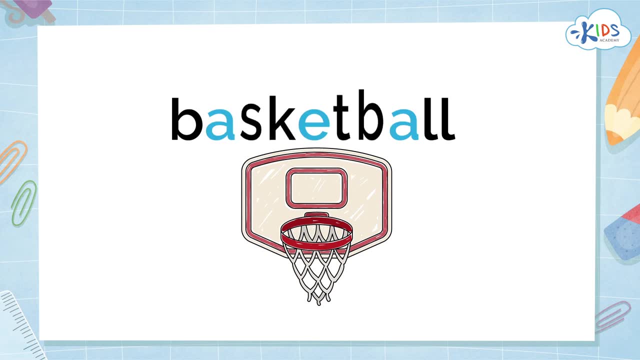 to decode longer words as well. Let's try this one. You can see that this word has three vowels, each separated by consonants, So it has three closed syllables: bas- and ket- and ball. This means that the vowel sounds are probably short: Bas-, ket-, ball. 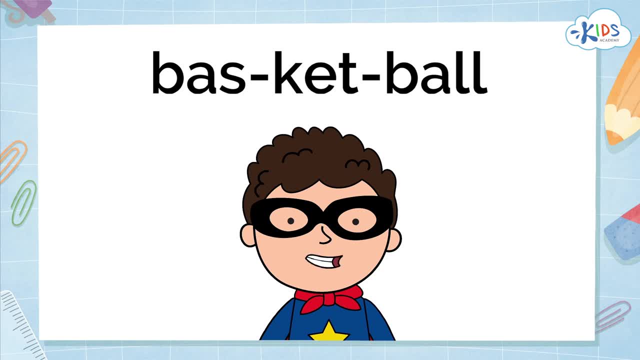 You can also check to see if you have divided the word into syllables correctly using this trick. Say the word out loud And place your hand under your chin. as you say it: Bas- ket- ball. See my chin hit my hand three times. So this word has three syllables. 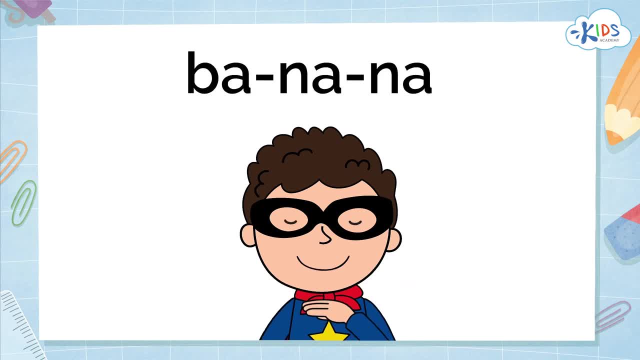 Let me show you one more. Try it with me: Ba-na-na, Three syllables. So the next time you come across a word that seems tricky, stop and look for syllables, Syllables, Syllables. See you soon. 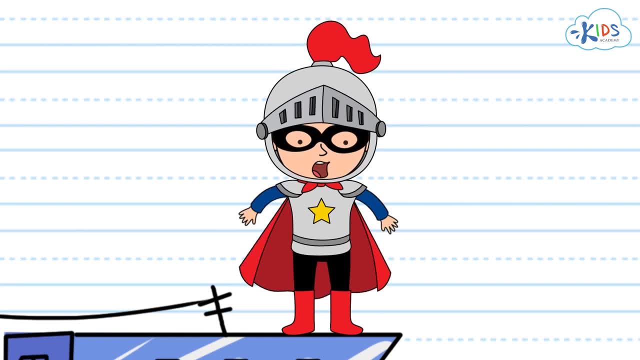 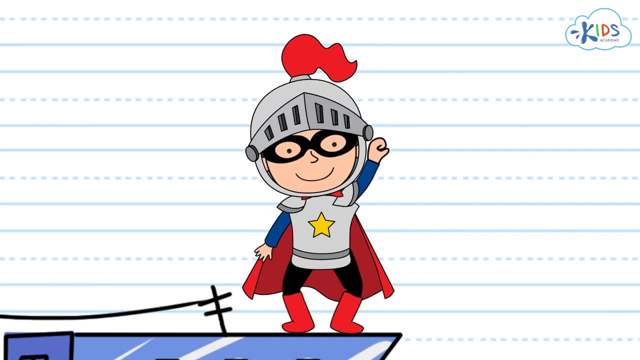 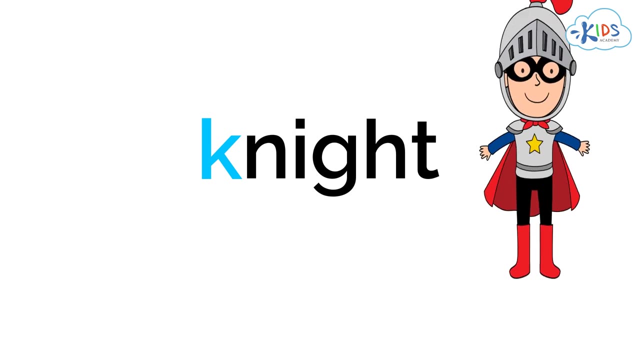 Hello, it is Chris, the Word Whiz, here with my super cool knight armor. Today we'll learn how to read words with silent letters. Take a look at that word, knight. Do you notice anything strange about it? Usually we begin figuring out a word by looking at the beginning letter. 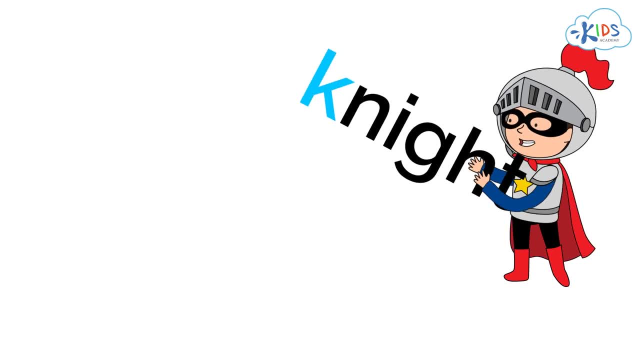 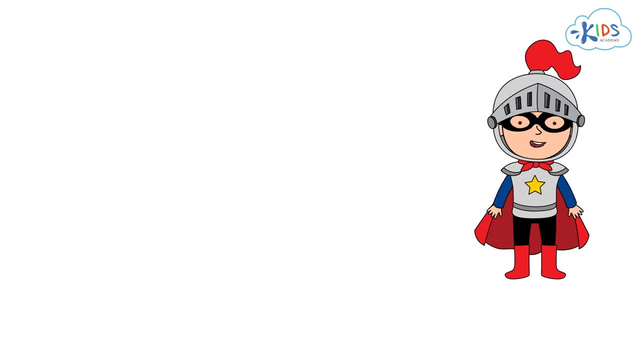 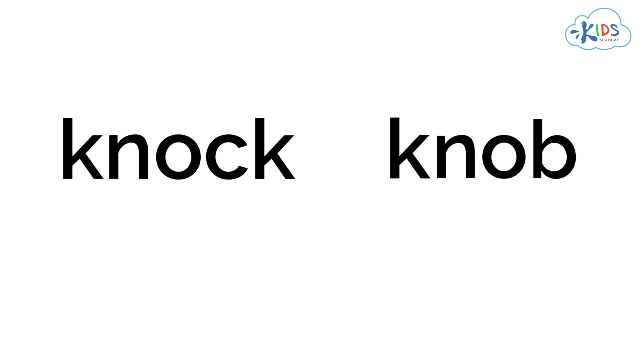 But that doesn't work here. This word breaks the rules. It is a jail word. Words like this with a silent letter are very tricky. Let's look at some more rule breakers. Here are two more words that begin with a silent K. 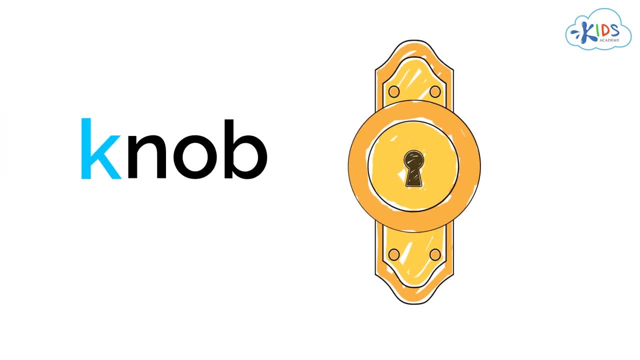 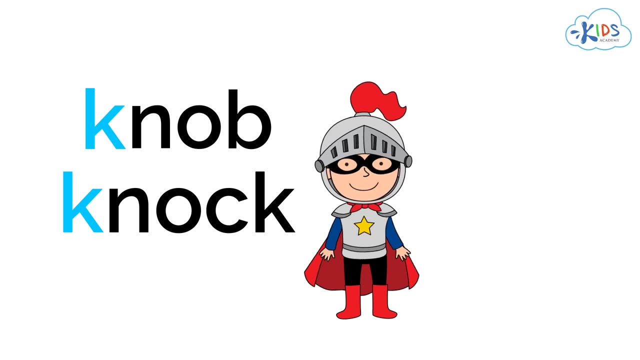 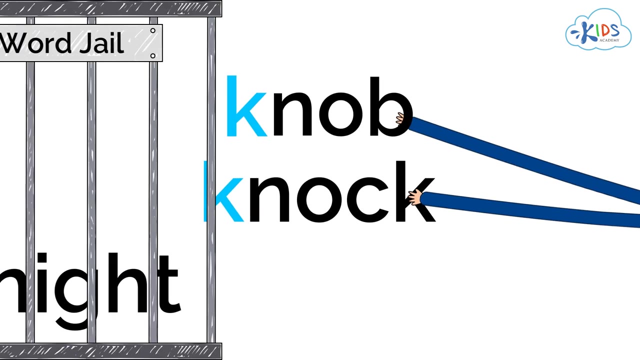 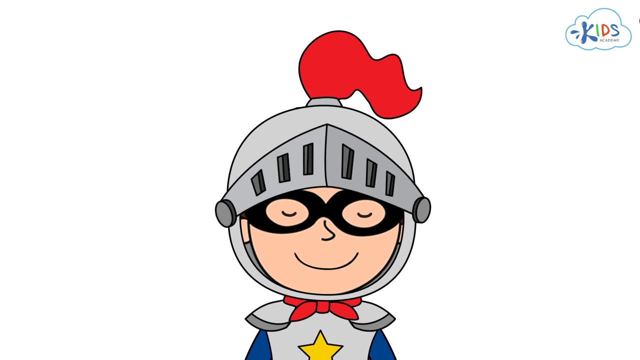 Knock and knob. We do not pronounce the K at the beginning of these words, Just like we do not pronounce the K at the beginning of night. These words break the rules, So I'll send them to the word jail too. There are other words that try to trick you too. 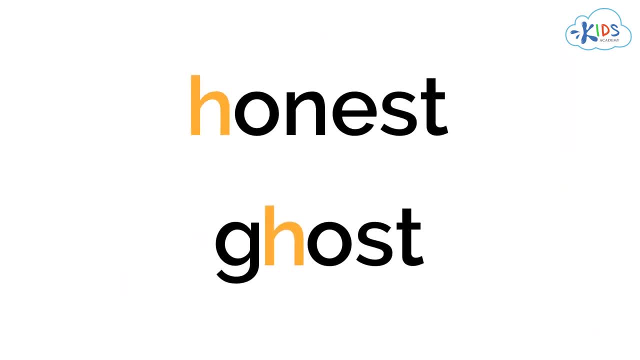 Check these out. In this word honest, we do not pronounce the H at the beginning. In the word ghost, the H is not at the beginning of the word, but we still do not pronounce the H sound. Now let's look at some silent B words. 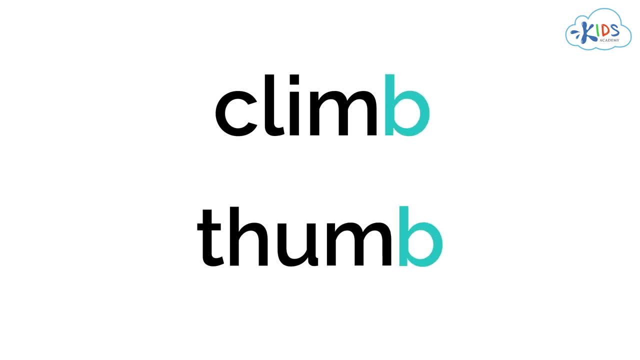 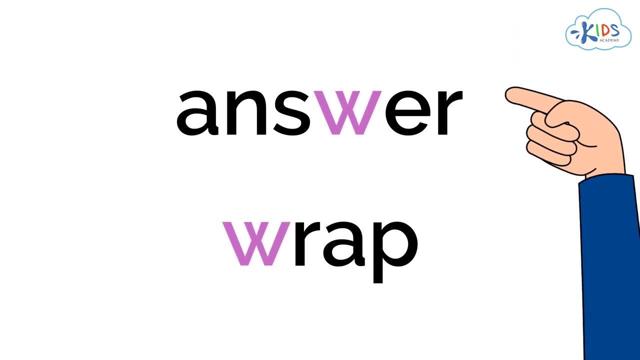 The B in both of these words is silent. We do not pronounce it Thumb Climb. The last silent letter we will look at today is the silent W like in answer and rap. Again, these words are tricky. They don't follow the rules. 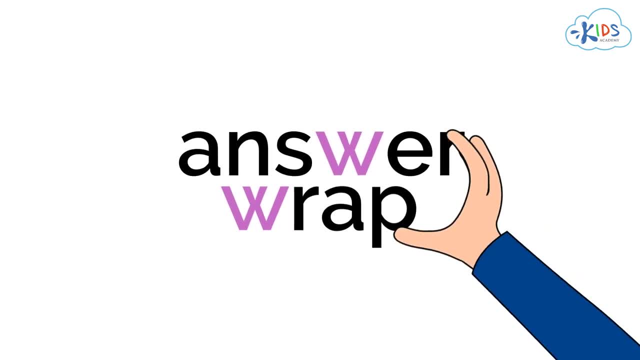 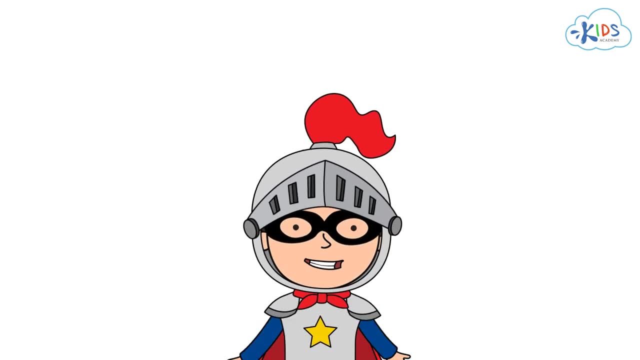 because we do not pronounce the W sound in either word. These are jail words too. Okay, are you ready to show what you know about those tricky silent letter words? Look at this word. Can you guess which letter is silent? That's right. 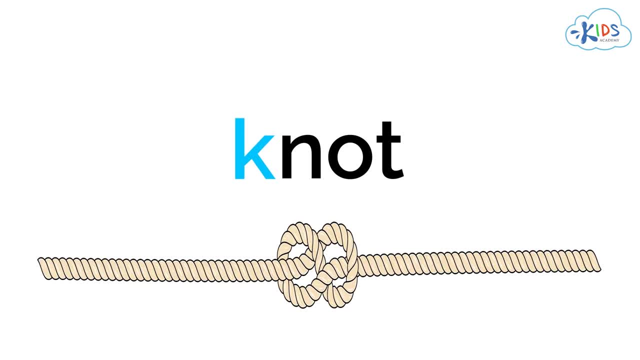 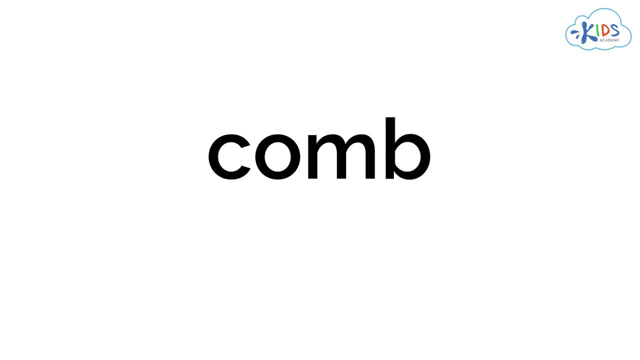 The K is silent. This is the word, not. Here's another one. Are you ready? Check this word out. Can you guess the silent letter? You bet That word has a silent B. It is the word comb. One more. 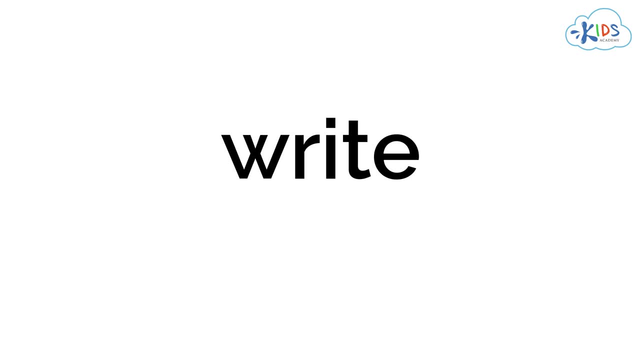 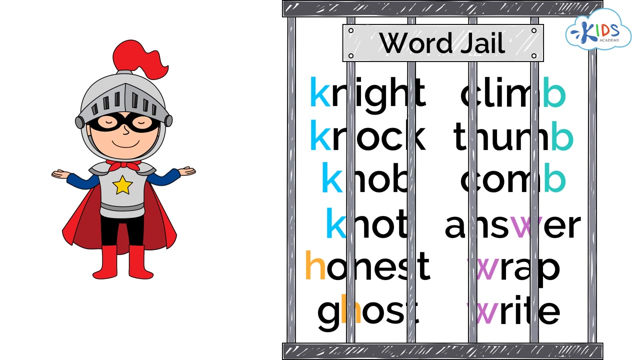 Don't get tricked. Can you find the silent letter in this word? Awesome job, There is no fooling you. This is the word right. Wow, There sure are a lot of tricky silent letter words. Good thing you have me around to throw these rule breakers into the word jail. 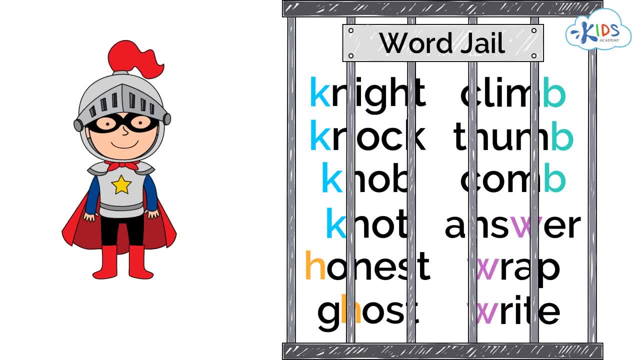 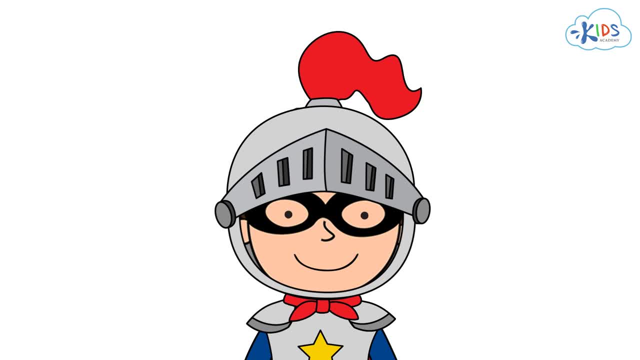 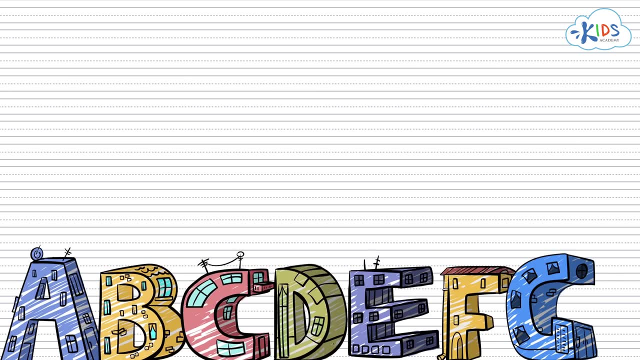 Don't let them trick you when you are out there reading. What other words with silent letters can you think of? Let me know in the comments below this video. See you soon. See you soon, Bye, Bye, Bye, Bye, Bye. 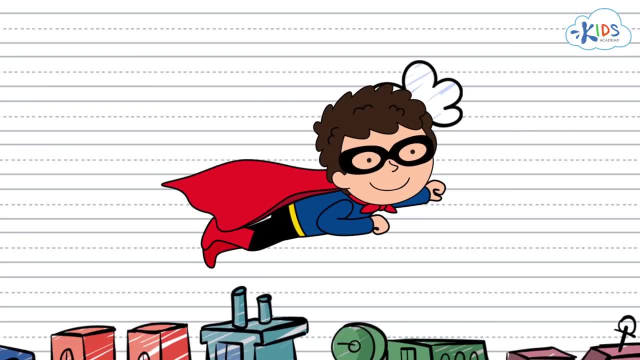 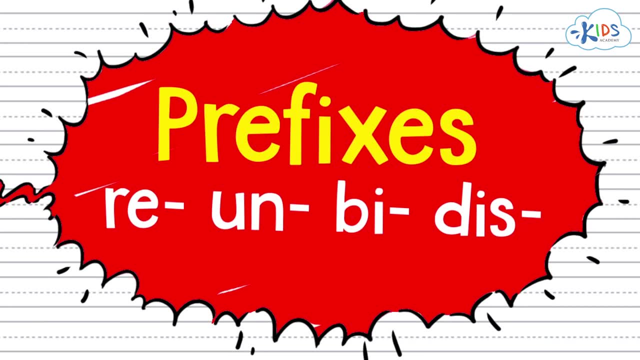 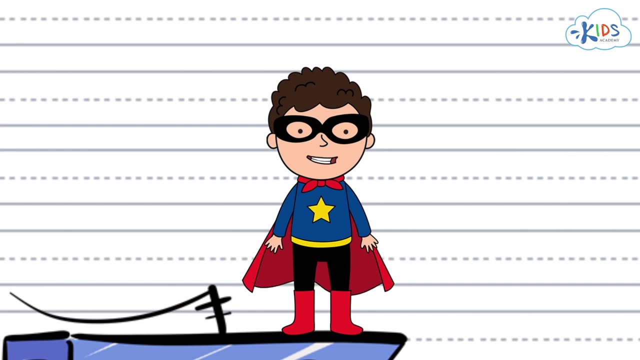 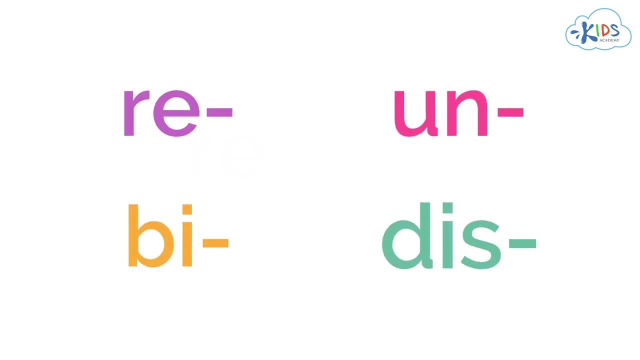 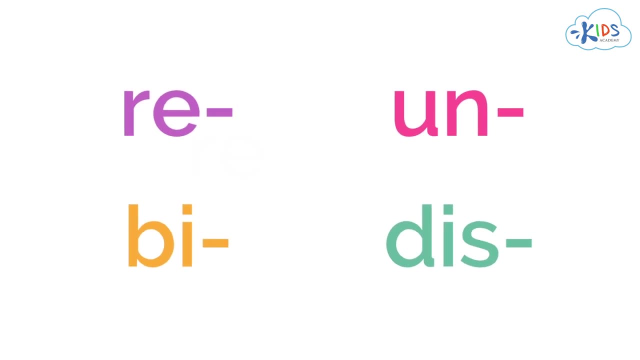 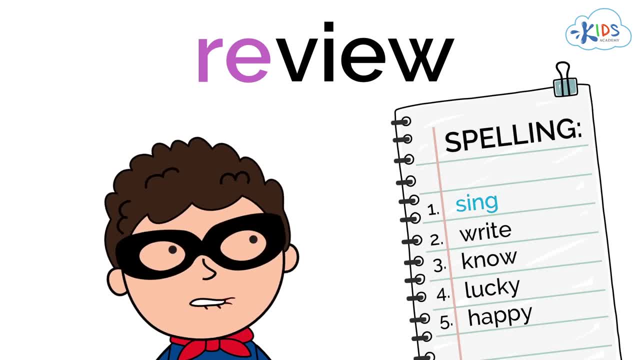 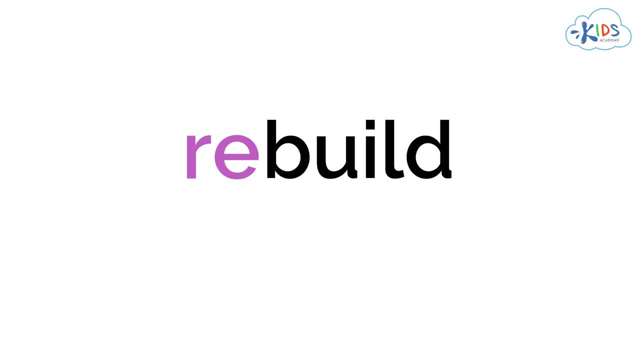 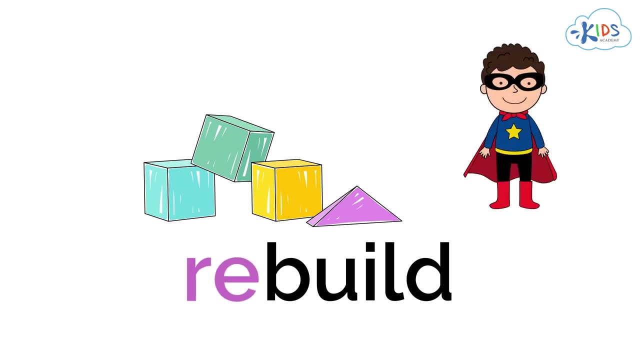 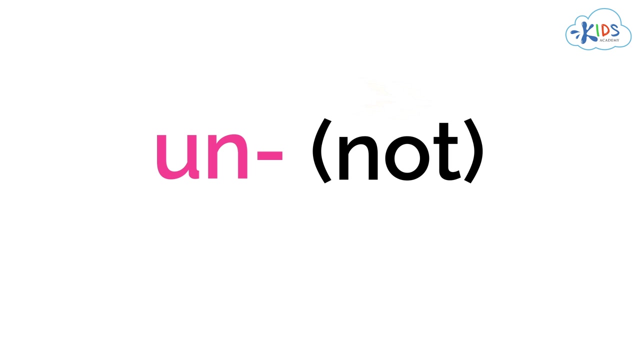 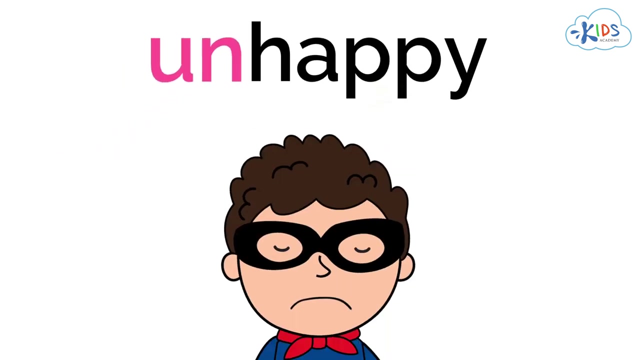 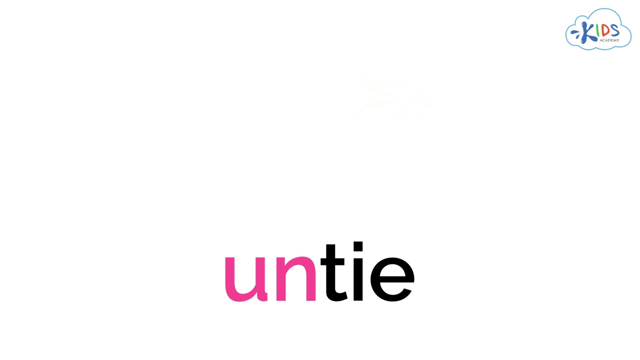 have. look at something again. we review words before a spelling test read build. let's look here. so we already know that. re means again. what does rebuild mean? yes, build again very nice. fun is another prefix. it means not like in. unhappy, that means not happy. here's another one. 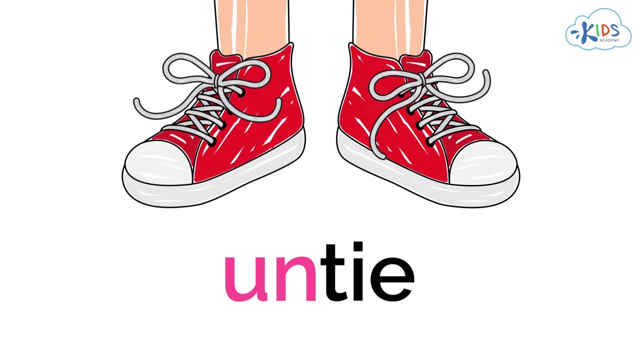 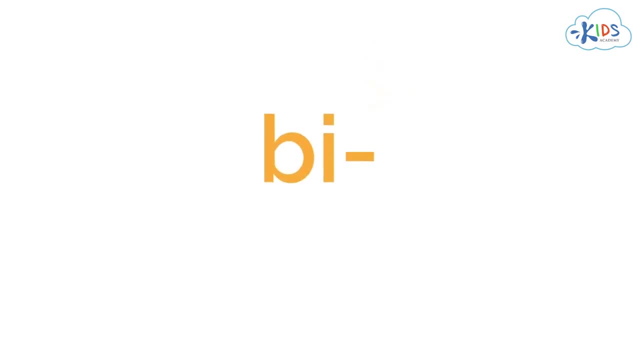 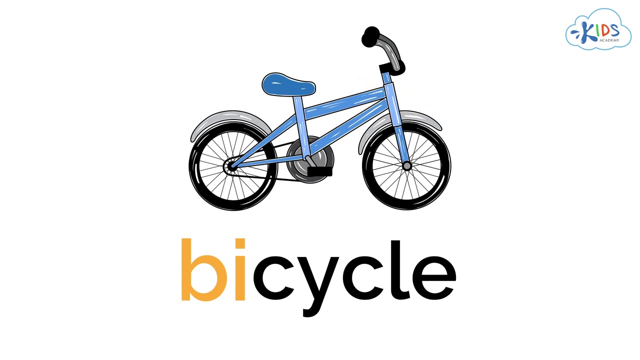 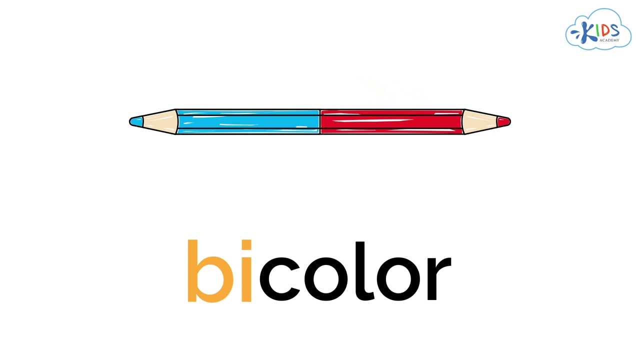 untie. a shoe that is untied would be not tied. let's look at by now I know that by means to do you think of bicycle? if we look at bicycle, it means there are two cycles or circles. bicycles has two circles for wheels. did you ever hear of by color? we know what color means if we have by. 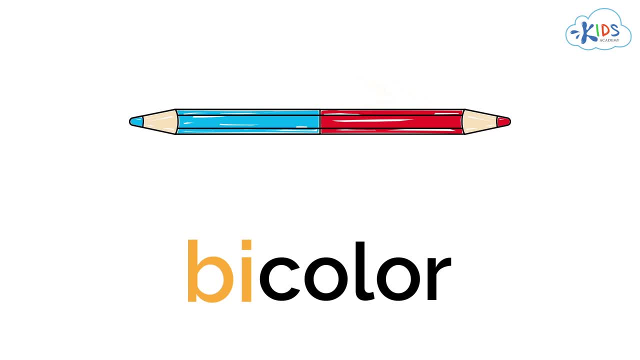 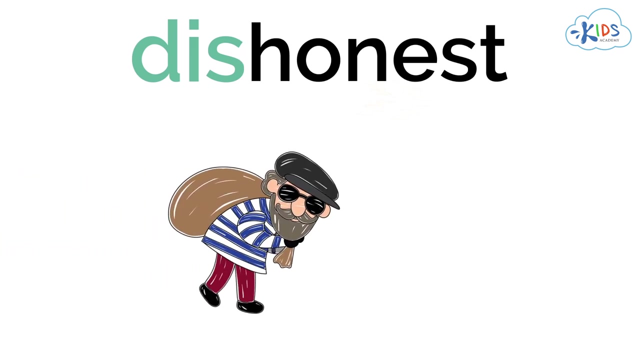 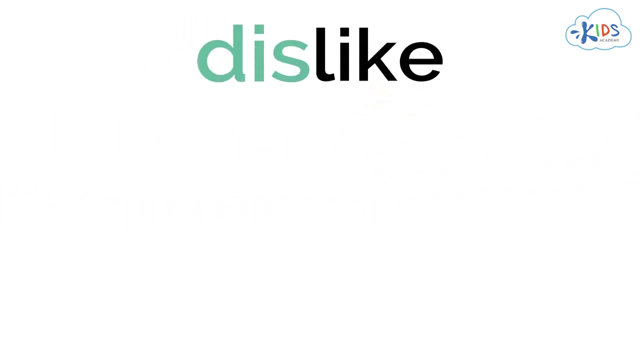 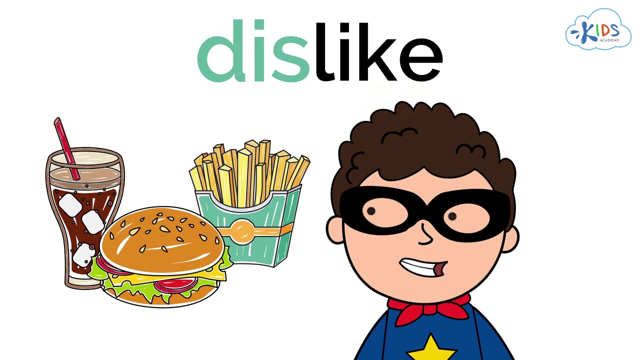 or two in front of it, it would mean two colors. the last one we will inspect today is dis. when dis is in front of a word, it can mean not. so if we say he is dishonest, we are saying he is not honest. take a look at this: dislike. what does that mean? yes, it means to not like. 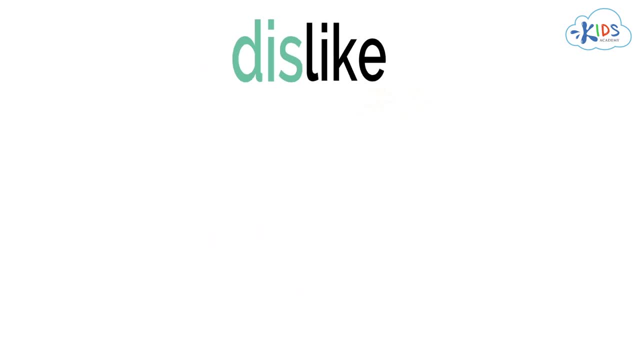 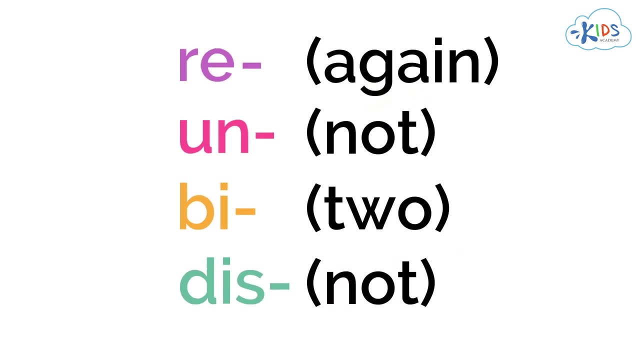 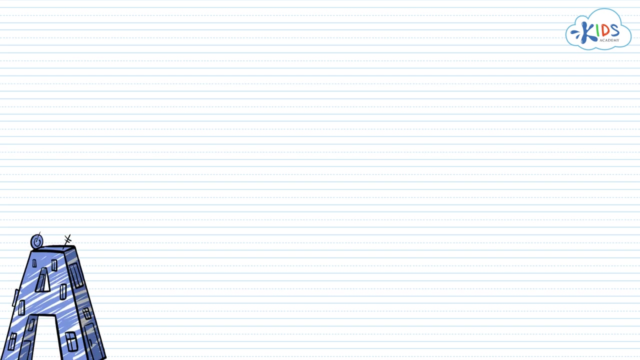 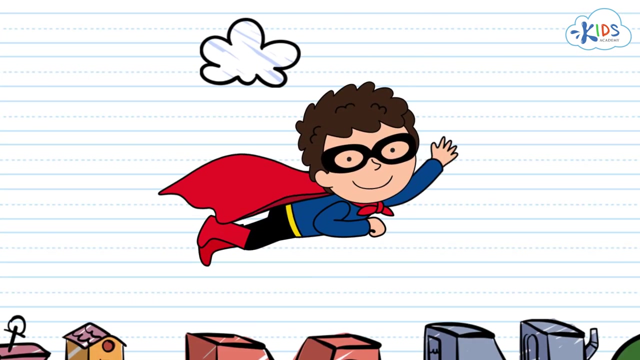 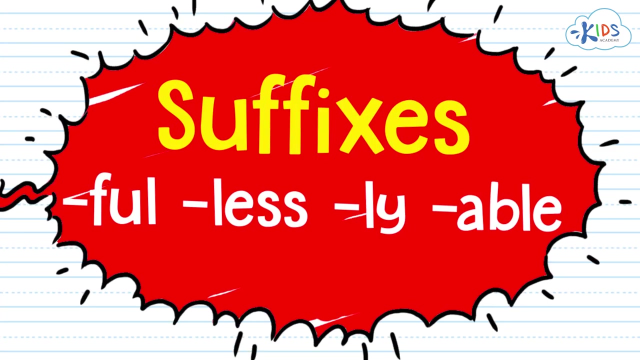 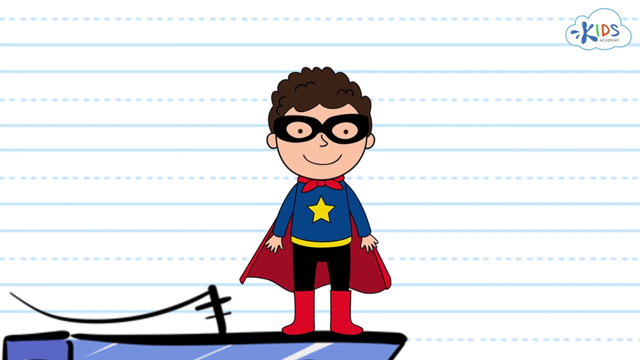 something nice work. you know four prefixes. I bet you will see many of these words now when you are reading. bye for now. hello, I am Chris, the word Wiz. we will look at the end of words today. are you ready to look carefully? let's go. suffixes are letters at the end of a. 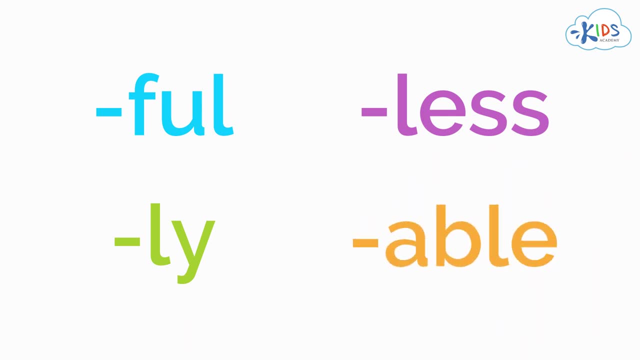 word. these change the meaning. we will look at four suffixes: full, less, leave and never read. this is the last one. there's two words talking. only three people have been reading four of these words today. are you ready to look carefully? let go suff. corpses are letters at the end of a word. these change the meaning. should I? had even coffee. three and four, my barrier. what was that say? what does it mean to say that's correct or do you have about 500 of them? messs with it. starting at end of our's heart. great mean verb: Explorer, we055 word. until now black and blue and 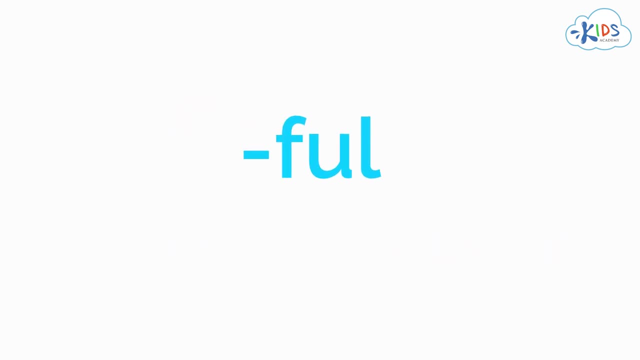 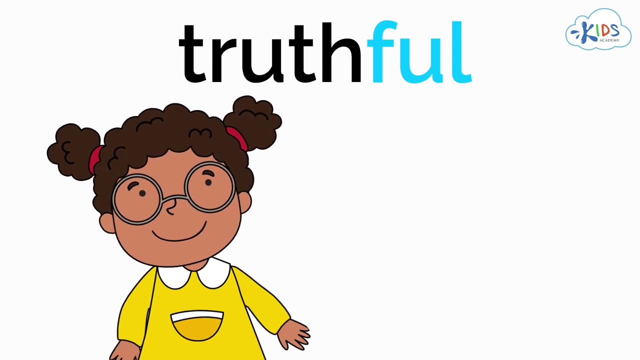 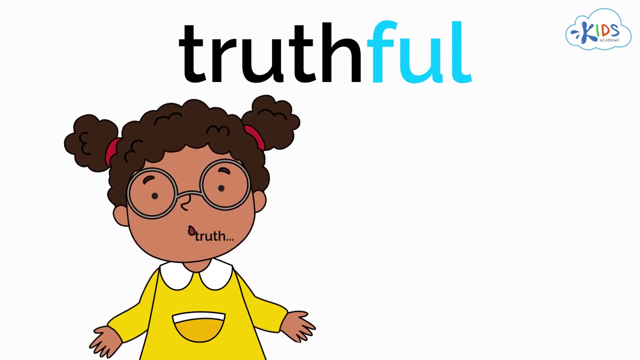 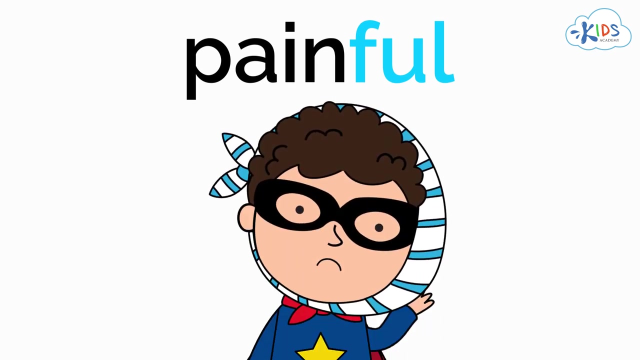 a bull. Here's one: Truthful. When we add full to a word, it means full of, just like it sounds. So truthful would be full of truth. If you are a truthful person, you are full of the truth or you tell the truth often. How about painful? What do you think that would mean? 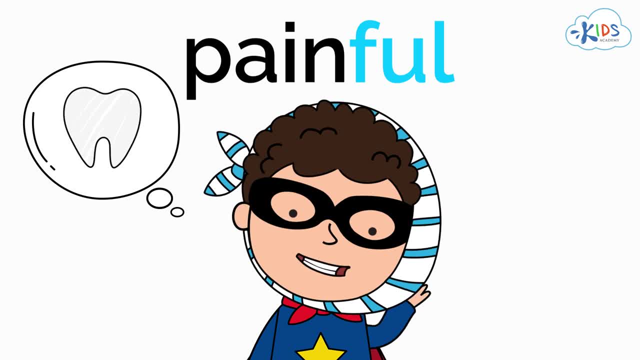 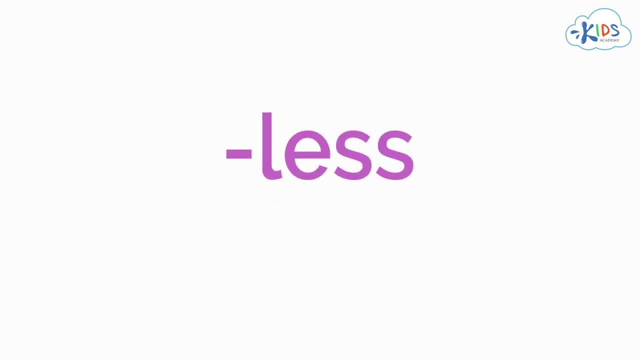 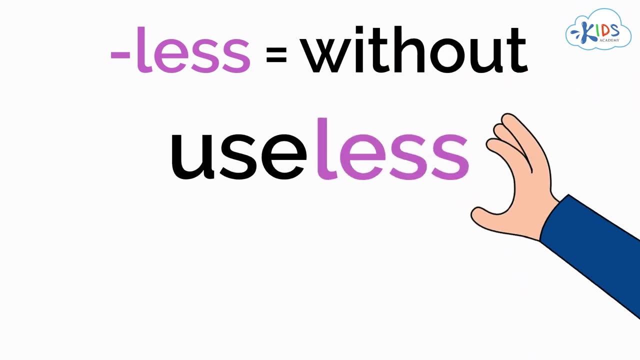 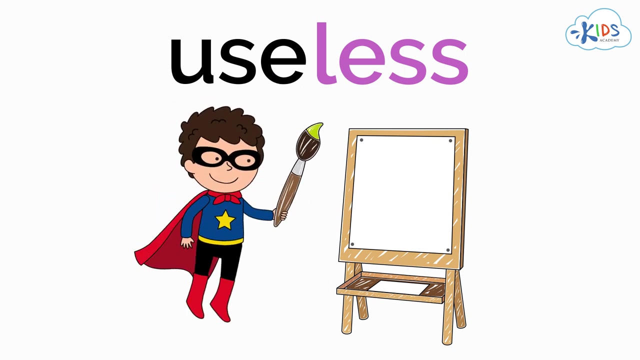 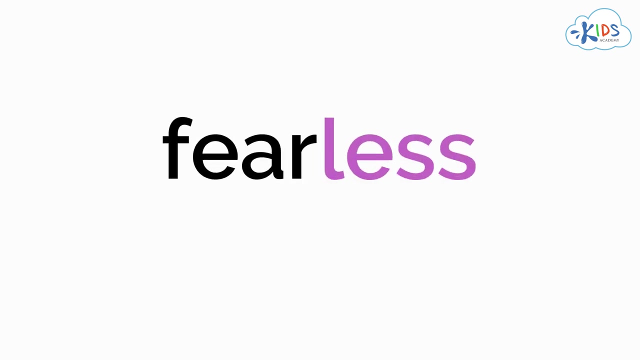 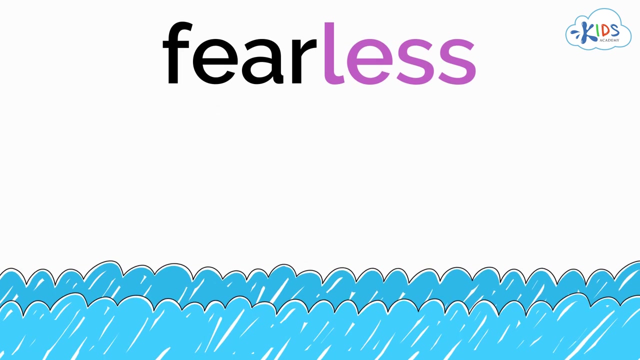 Yes, full of pain, Ouch. Another suffix is less. This means without. So if we had use and added less, it would mean without A use. A hammer is useless for this project. It is without use for this. Let's look at fearless. Less means without, So this would mean without fear. 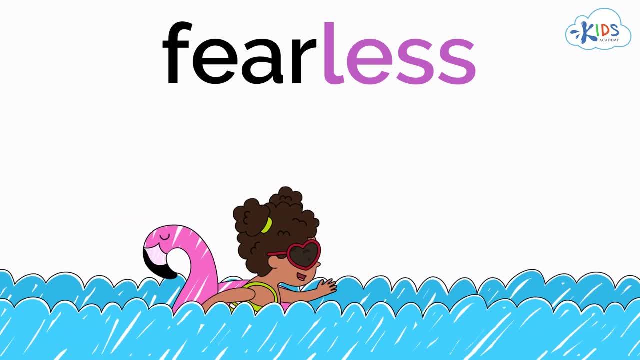 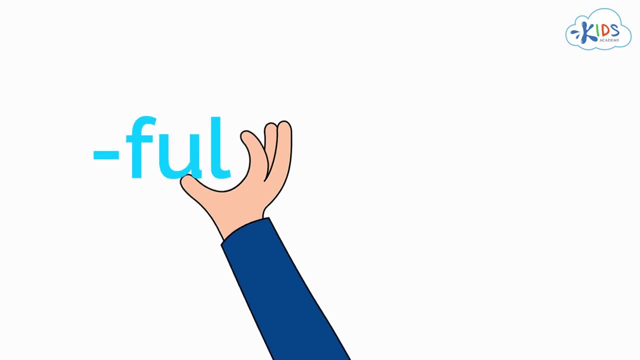 She was fearless when she swam. She was fearless when she swam in the ocean, So she wasn't afraid. We looked at full and less. Our third suffix is lee. This one is a little trickier but I know you can handle it. 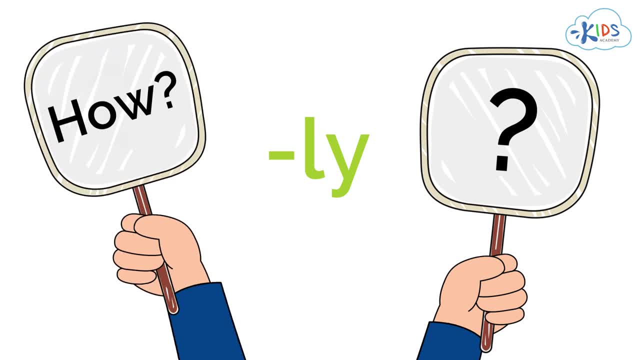 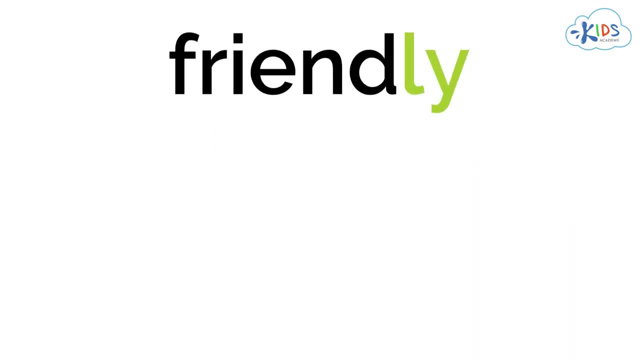 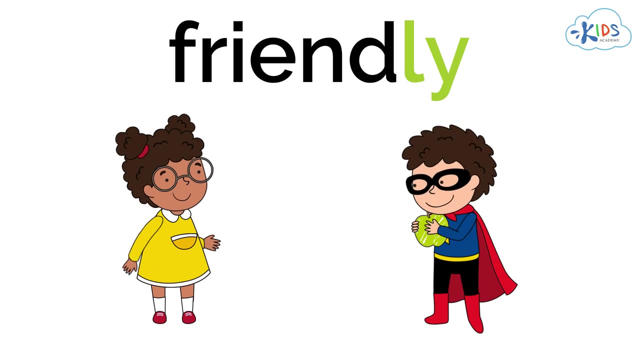 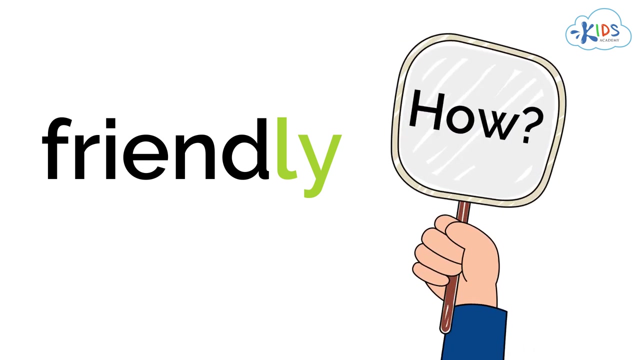 Lee answers the question. how Sometimes it answers the question. how often You can try this one? She acts friendly to everyone. What question does it answer? How does she act? You got it, She is friendly. Let's look at another word with lee. 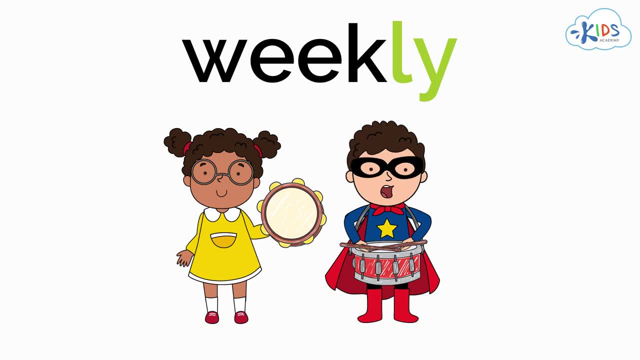 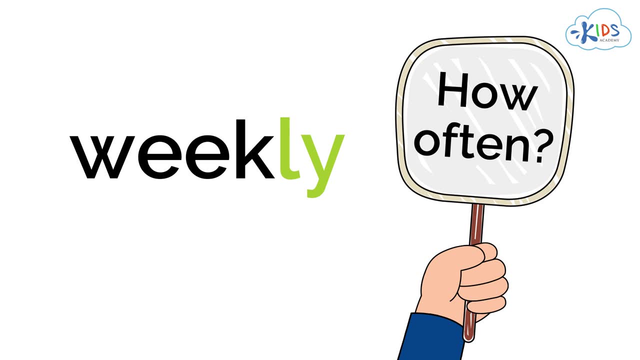 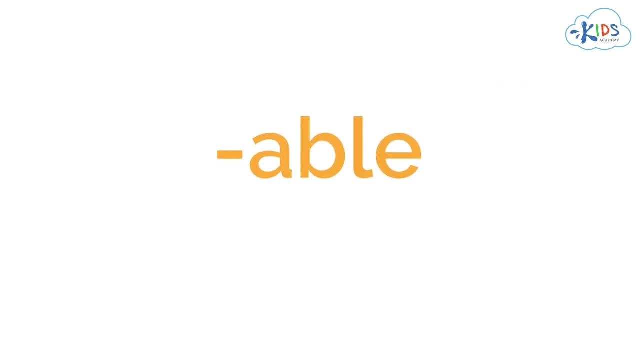 The class has a weekly music lesson. This answer the question how often A weekly lesson would happen once a week. We have one more suffix for today: A bull. It means you can do something. It looks like the word able, But as a suffix we say a bull. 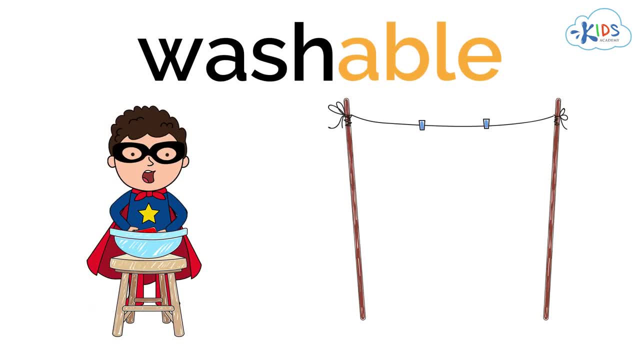 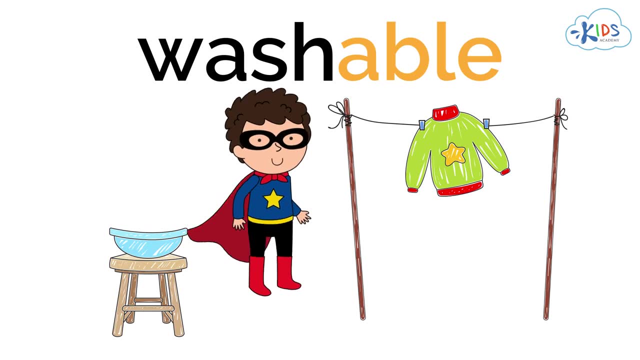 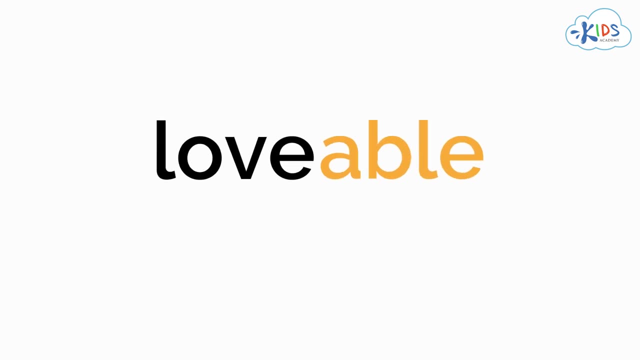 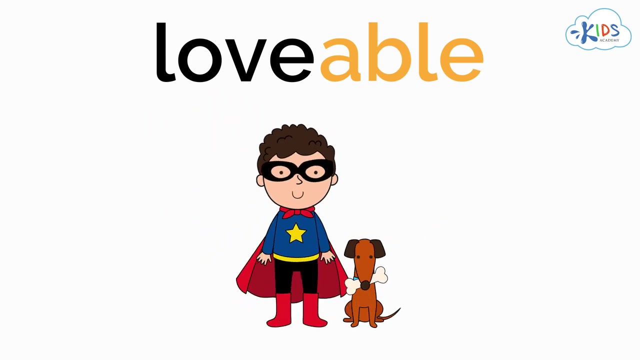 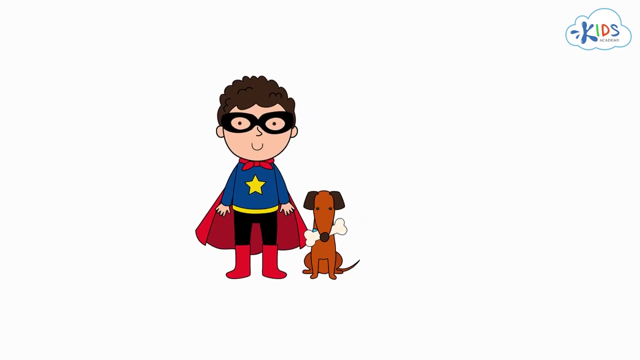 a bowl, like in the word wash a bowl. a washable sweater would be a sweater that can be washed. hmm, what about lovable? the dog is lovable. what would it mean? yes, you can love the dog. nice work, you know four suffixes. i bet you will see many of these words now when you are reading. bye, for now. 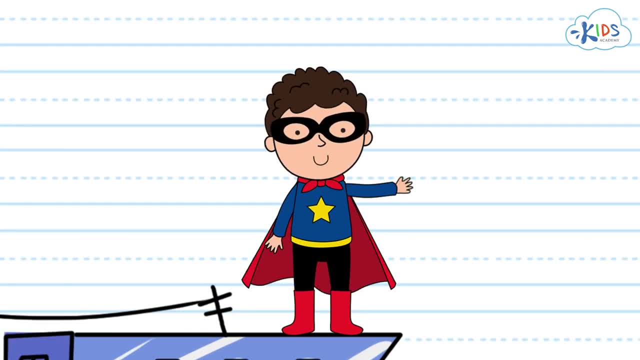 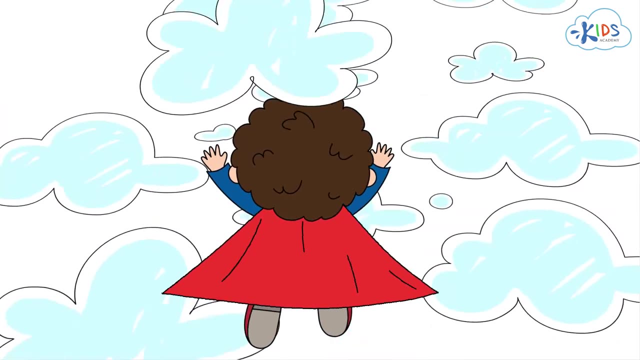 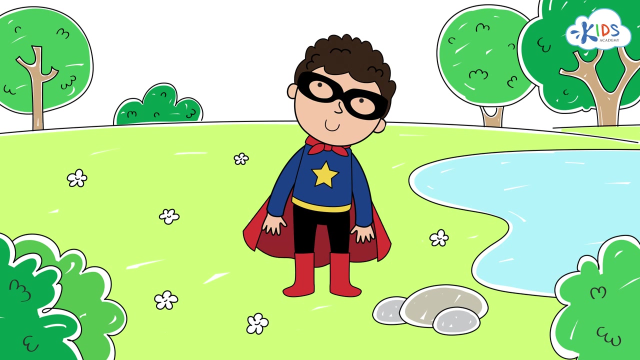 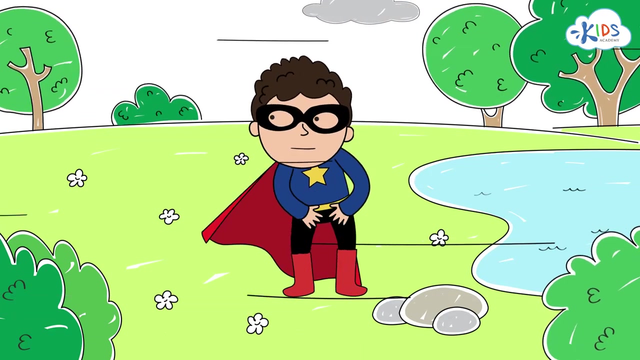 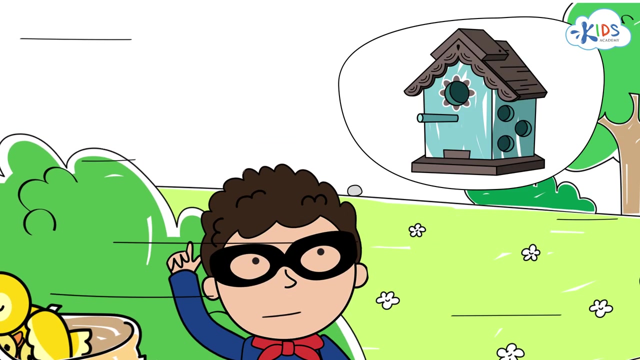 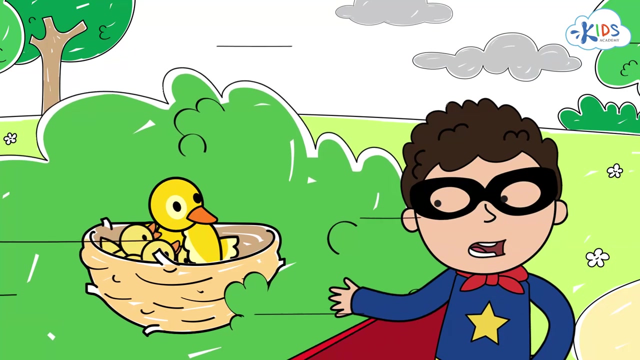 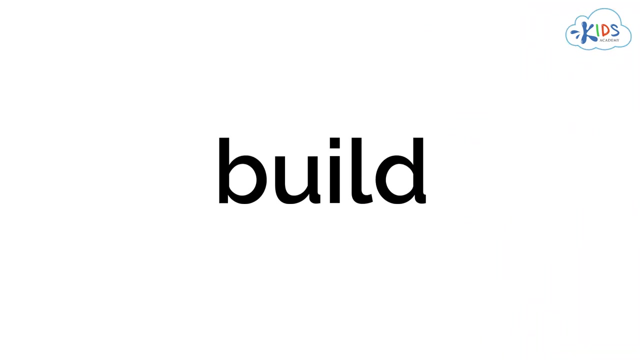 so, hey, friends, today i'll tell you what parts can be found in a word and how suffixes and prefixes help us build new words. let's go so. we need to build a house for these little birds or they'll catch a cold. build is a verb. if we add the letters er to it, we'll get the noun builder. 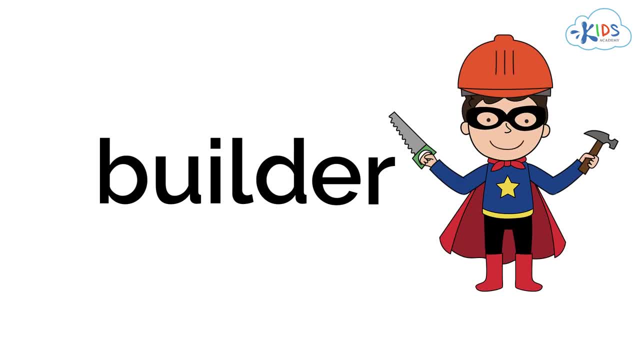 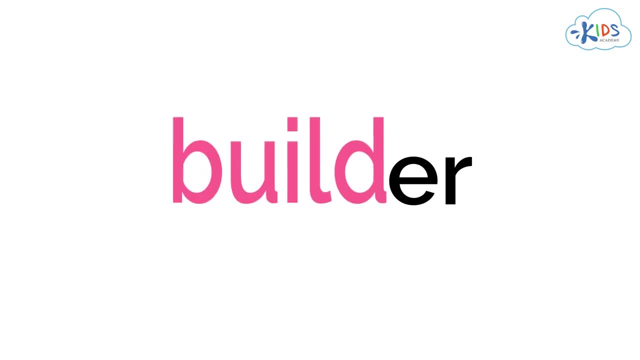 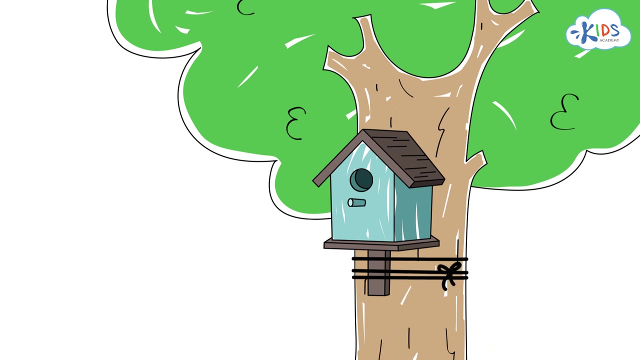 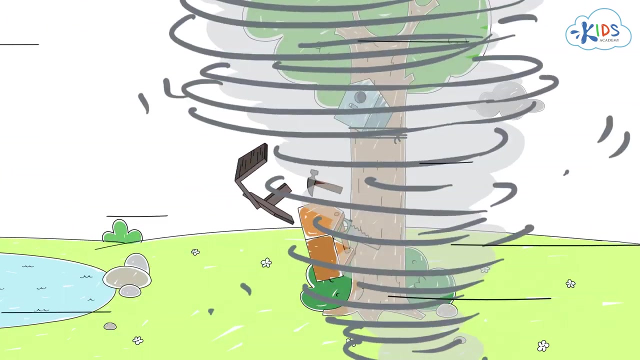 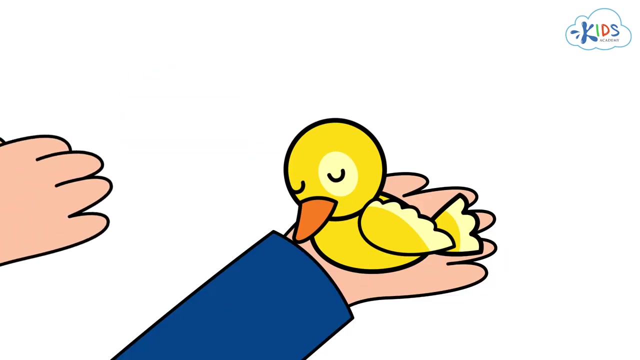 which means a person who builds something. in the word builder, build is a base word and er is a suffix. a suffix is added at the end of a base word and changes its meaning. that's where it comes from. so we'll get er build. no worries, we'll rebuild the birdhouse. 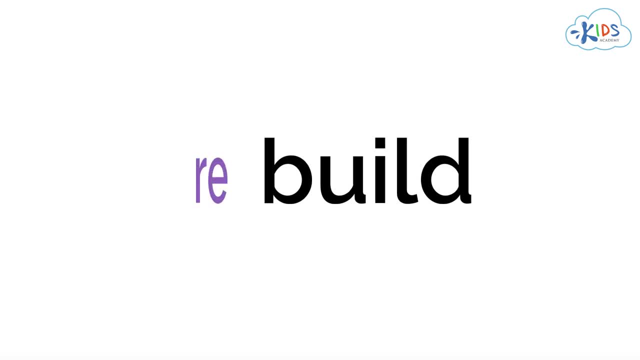 if we add the letters r, e in front of the base word build, we'll get a new verb, rebuild, which means to build a house, To build something. again, Re- is a prefix. It helps to create a word with a new meaning too.